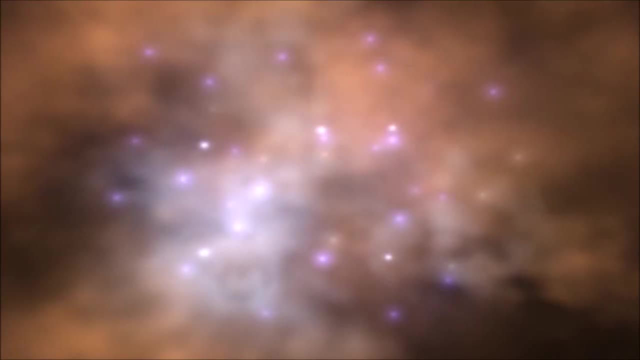 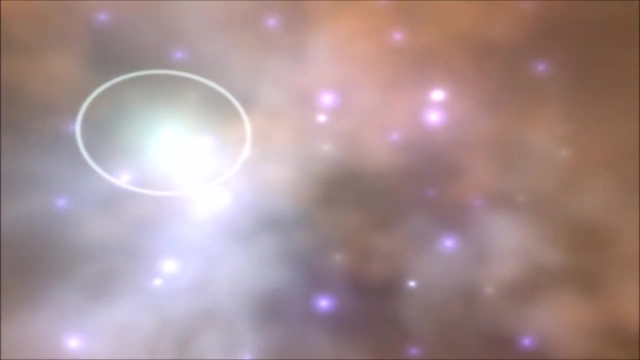 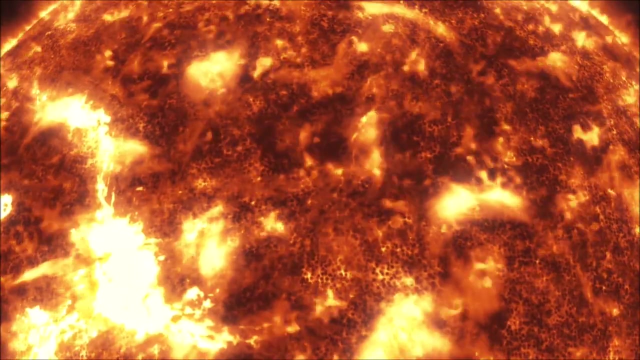 and denser. Once the core is hot enough and dense enough, fusion kicks off and the hydrogen gas begins to turn into helium, A star that is fusing hydrogen is not a protostar any longer, but has entered something called the main sequence- The life of a star on the main. 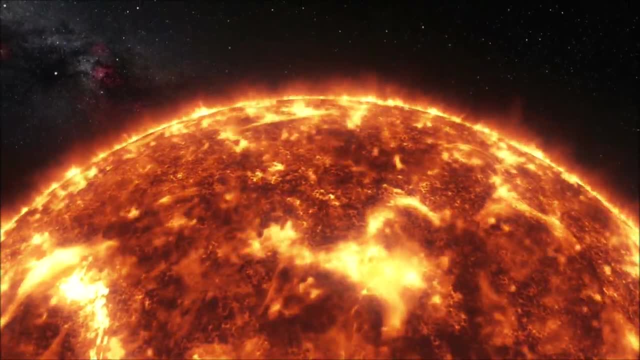 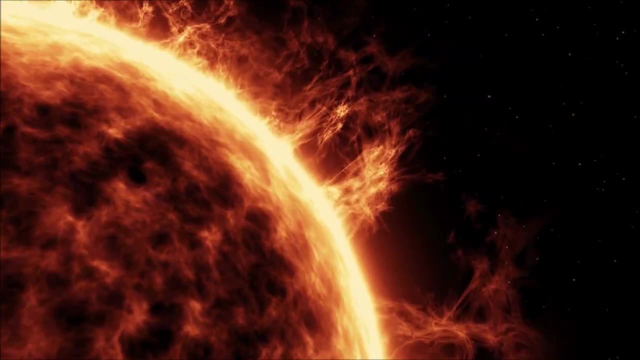 sequence is a constant battle against gravity. Stars are so massive that if gravity was the only force working on them, they would collapse immediately. Fortunately, stars have super-hot cores that create a huge amount of heat, which is why they are called protostars. They. 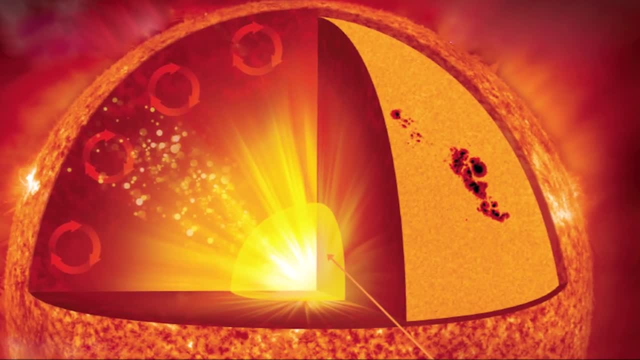 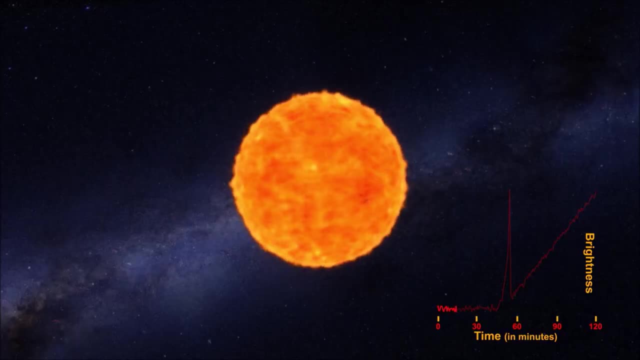 create pressure and work against gravity, producing a state of equilibrium. The star will be okay as long as the force of gravity pulling the gases inward and pressure from the core pushing the gases outward are in balance. Eventually, however, the star 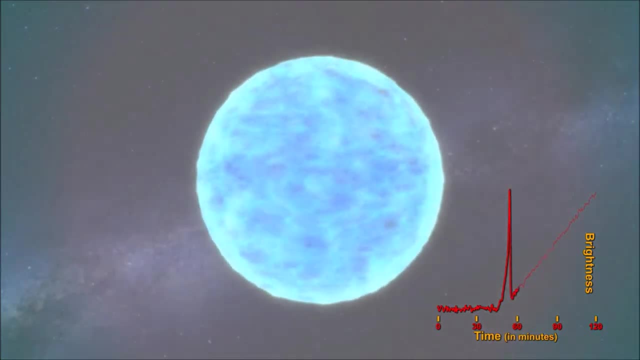 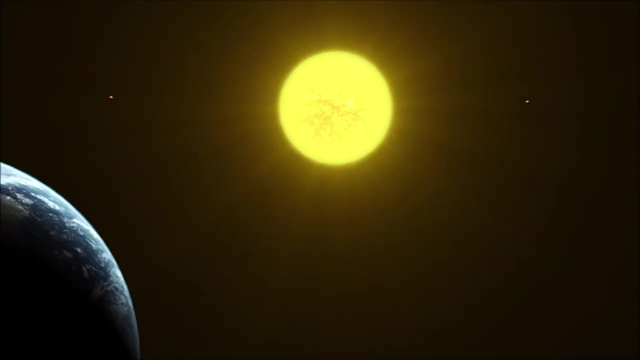 will run out of hydrogen to convert into helium, and when that happens, gravity wins. The inner layers of the star begin to collapse, increasing heat and pressure at the core. When the core expands several hundred times their normal size, the star becomes a red giant. Meanwhile, 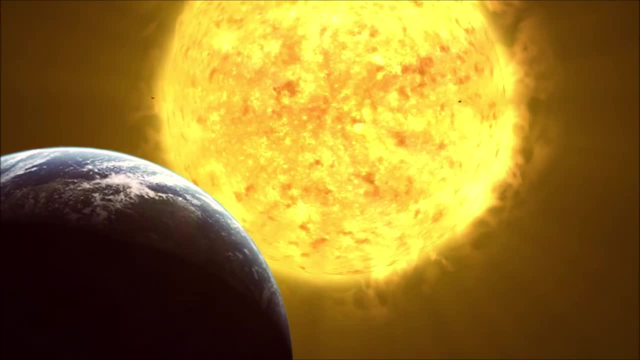 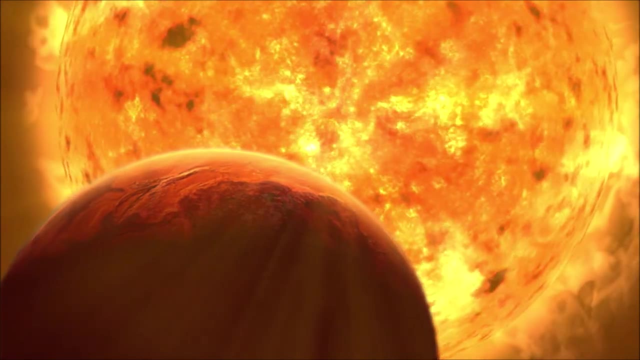 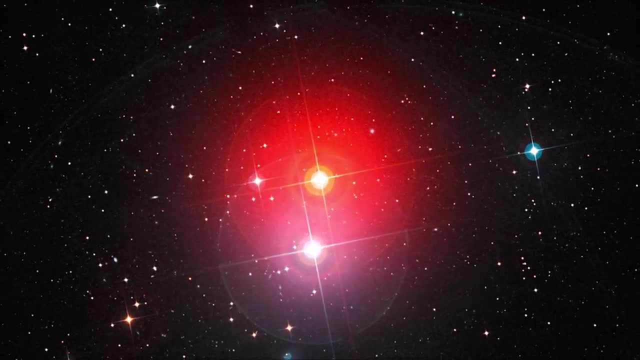 the outer layers expand several hundred times their normal size and the star becomes a red giant, Or, if the original star was massive enough, a red supergiant. When a medium-sized star becomes a red giant, there is temporarily enough heat and pressure. 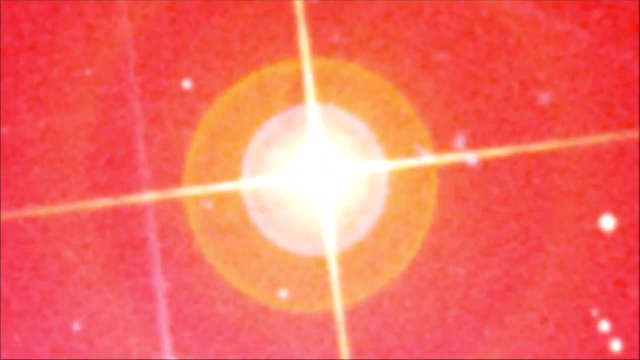 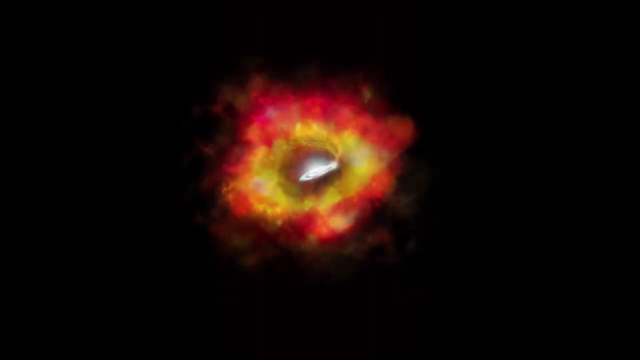 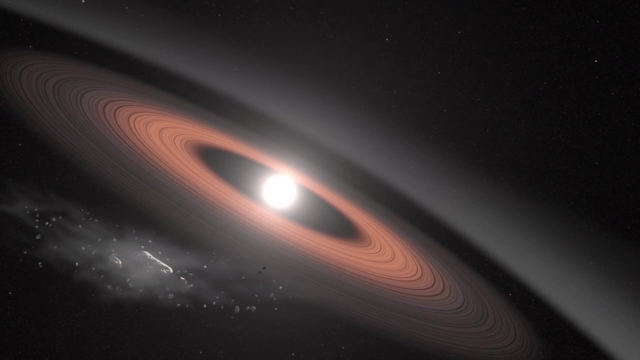 in the core to fuse helium into carbon, preventing further collapse. Once the helium and the helium are gone, however, the core collapses again and the outer layers of the star are blown away. The collapsed core becomes a white dwarf, a dense, slowly cooling remnant about the 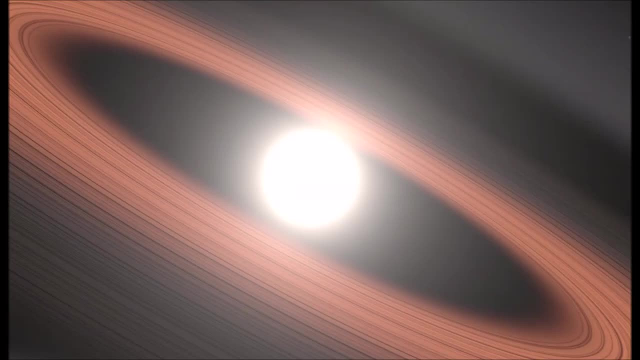 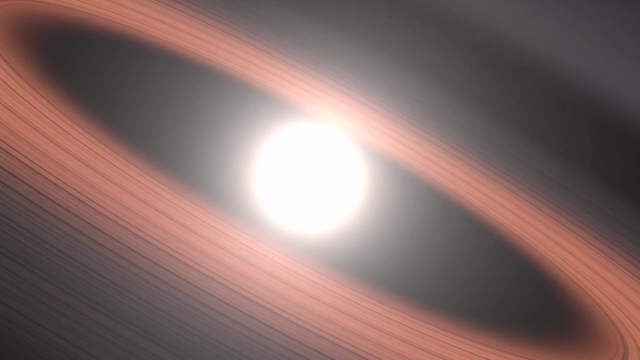 size of a planet. The atoms in a white dwarf are so close together that it simply cannot collapse anymore. But once the stored heat in it is gone, it will no longer glow and will become a black dwarf spinning darkly in space.